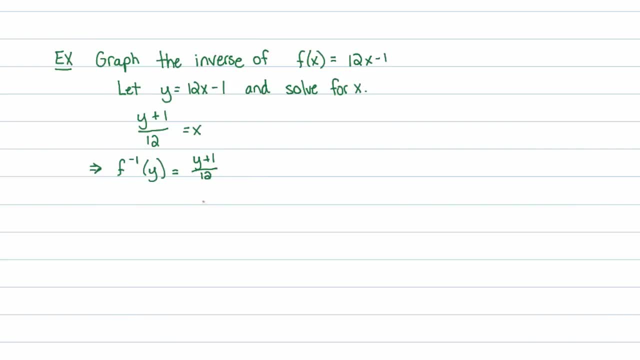 to y plus 1 over 12.. And I told you in my last lecture that I appreciate and really like this form of the inverse function, except in one case, And that one case is when you're asked to graph. When you're asked to graph, you should swap this variable out, Call it. 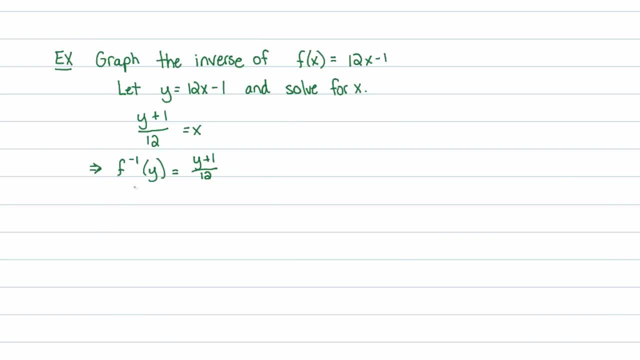 a different letter. In fact, call it x. The reason why is because when we're graphing, we like to use our inputs along the x-axis and our outputs along the y-axis, So in this case, I'm going to go ahead. 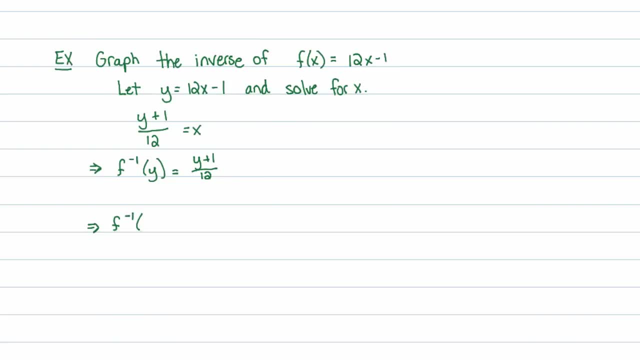 and just call my inputs the letter x And just tell you right now, this is not the same x as this one up here. It's not the same one, So that's what's so confusing about it. By the way, this can be written as x over 12 plus 1 over 12, if you wanted to write it. 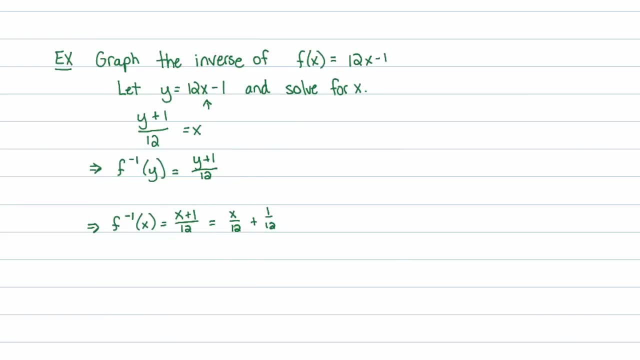 that way, which I do. And let's go ahead and graph this function, And there's a couple ways you could do it. You could just graph it. Actually, now that I'm thinking about it, there's three ways to graph the inverse of this function. I could use the fact that this is in y equals mx plus. 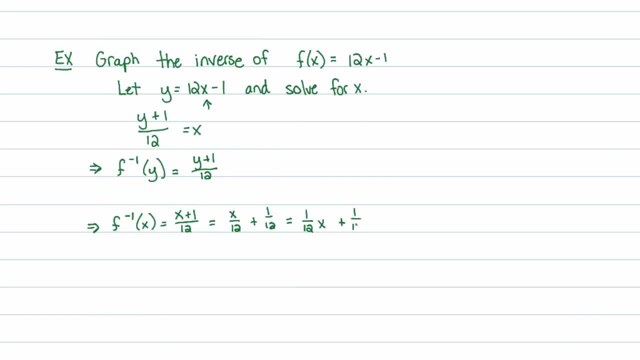 b form: 1- 12th, x plus 1.. plus 1- 12th. so the slope this is a line with slope 1- 12th and y intercept of 1- 12th. i could do that or i could build a table of values. that's. that's another way i could do it. so, um, if i want to build, 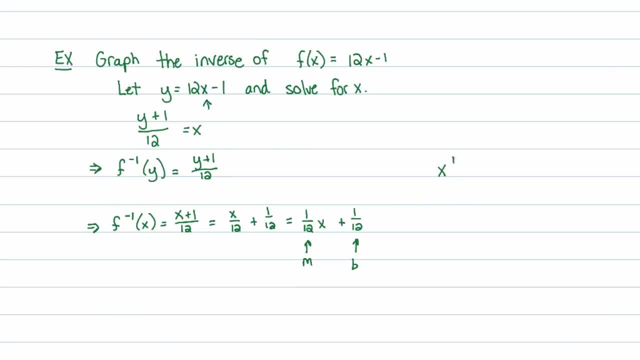 a table of values. looking at this f inverse function, i'll probably pick smart values for x, like x equals um. let's do x equals 11. 11 plus 1 is 12. 12 divided by 12 is just 1. and remember, since this is a line, i only need two points, so let me do a negative value for x as well. uh, let's do x. 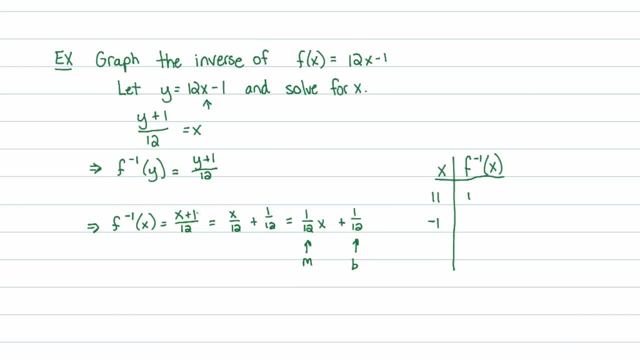 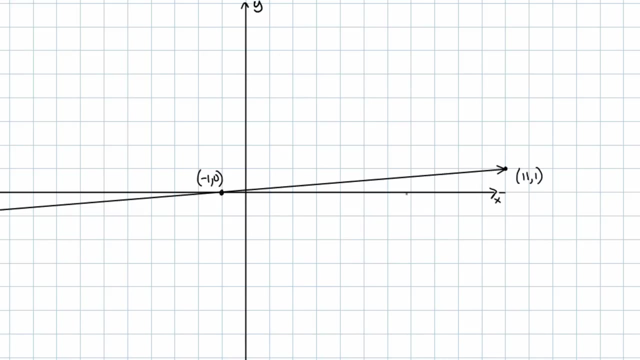 equals a negative 1. negative 1 plus 1 is 0. so there we go, all right. so these are my two points and i'll go ahead and grab my graph that plot those two points and graph that line. what i get is this line right here, very shallow line. now, what i'm going to demonstrate next is 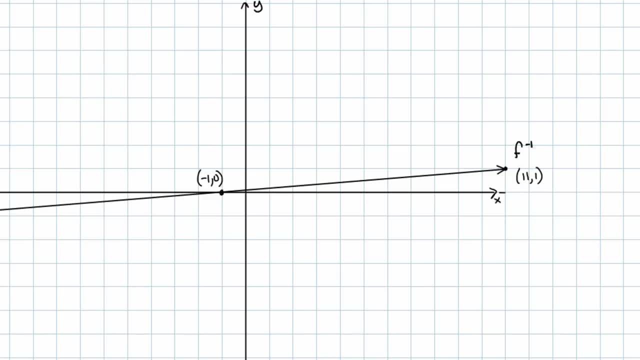 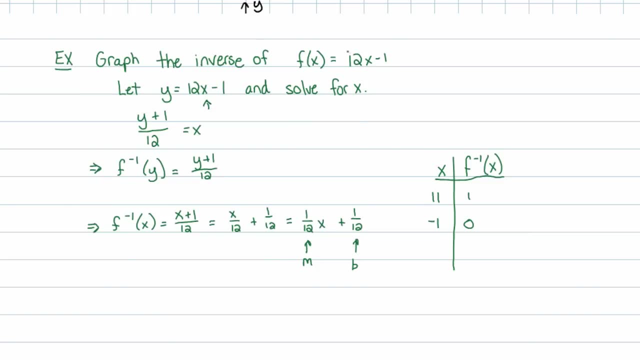 i'm going to use the original function. so this is f inverse of x here. i'm going to go ahead and plot f of x now to show you what f of x was. f of x was just 12x minus 1, so it's a slope of 12. 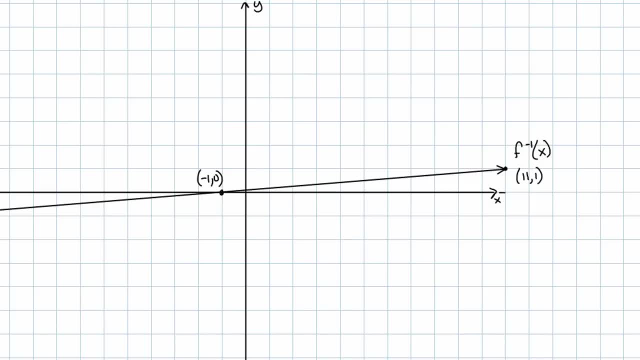 and y intercept of negative 1. so let me go ahead and plot the y intercept of negative 1, and then the slope is 12, so I'll go up 12 and over 1, 1, 2, 3, 4, 5. oh, this is going to all go off the screen. 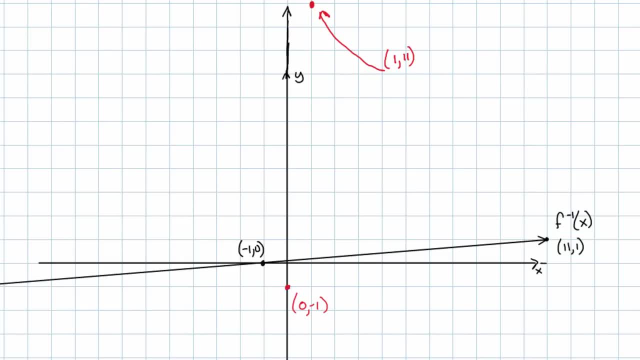 now. I don't know if you could see it, but I've already plotted, like I said, the y intercept zero comma negative 1. I've shifted the graph down here so I can make more room. but the other point is 1 comma 11, rows 12 went up and i'm going to plot: ahiccp rushed out of that 1 çıktı and barillä 5: 1. 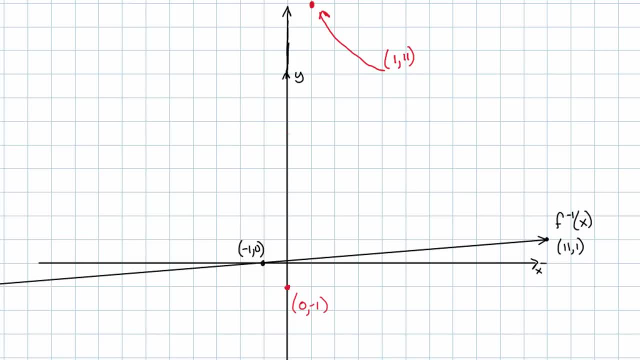 0 comma 0: 1, but the other point is 1 comma 11. i number has 1, she 12, and i've shifted the graph down here to see if there's anything. 12 went over 1, but if you rise 12 from a height of negative 1, then you go up to a height of 11. 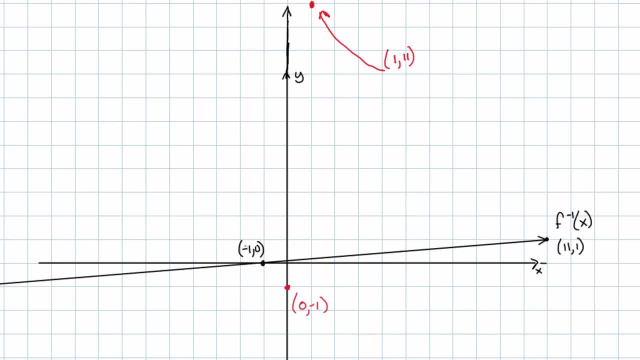 and then over 1. notice something about these x and y values. look at this: the x value here is negative, 1, the y value is 0, and look at here they're swapped. look at this: here x values 1, y values 11, and here they're swapped, of course, because they're inverse functions. so the x and 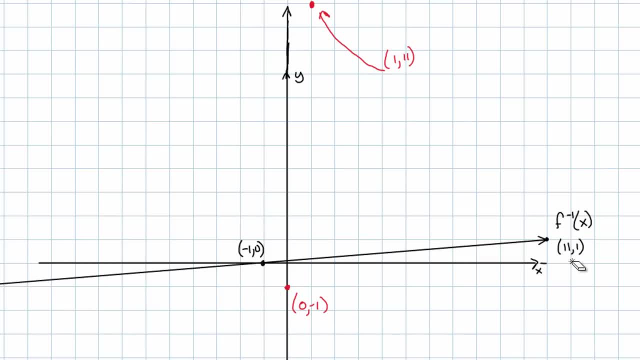 y values play opposite roles. they're swapped in these. in this case, let me go ahead and draw the line in, and so that is the line for f of x. that's that's the graph of f of x. there's something i want you to notice about that, since all the x and y values are swapping across those two lines. 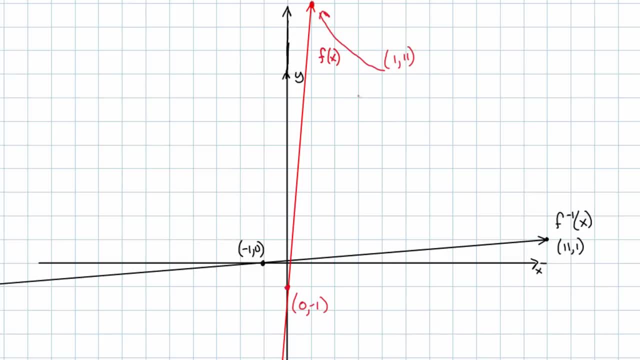 that means that it should be a reflection about the line y equals x. like that, it should be a reflection about the line y equals x. and if you look at these two graphs, the red graph and the black graph, they sure are. they're absolute reflection about the line y equals x. it's because once you're about that line, if you 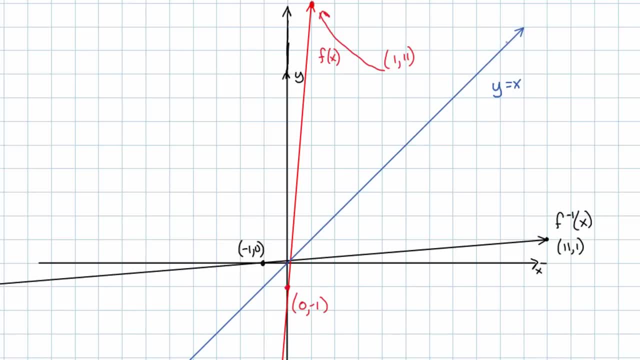 consider the world around that line: y equals x. well, that's where y is the same thing as x. but on, let's say right here this point: it's x and y values are opposite the x and y values there. in fact, let's see, that's one, two, three, four, five, six, seven, eight. that's x equals eight, y equals one. 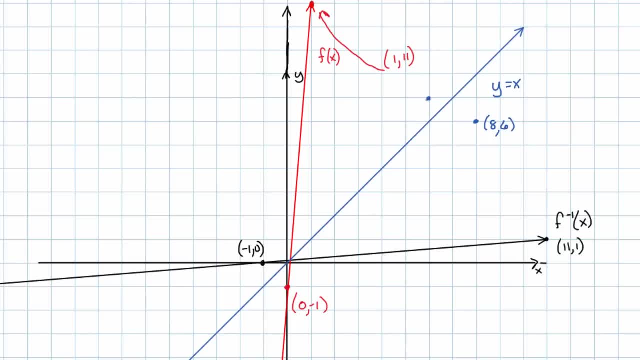 two, three, four, five, six. and this point here is actually, since it's two back, it's x equals six. and well, i must count it wrong. nope, wasn't that i counted wrong. it's that i put the point in wrong spot. this is the mirror image right there. anyway, it's two back, that's x, value six. 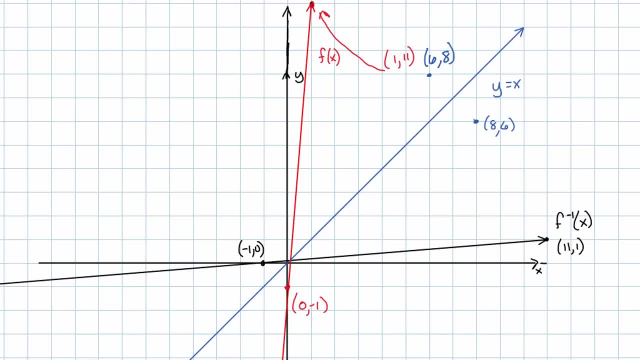 and two up, so we were at a height of six, we're now at a height of eight. see, these two are mirror images about this line. y equals x here, and their x and y values have been swapped. that is true for every point on the coordinate plane. pick any point that you want and pick its mirror image. 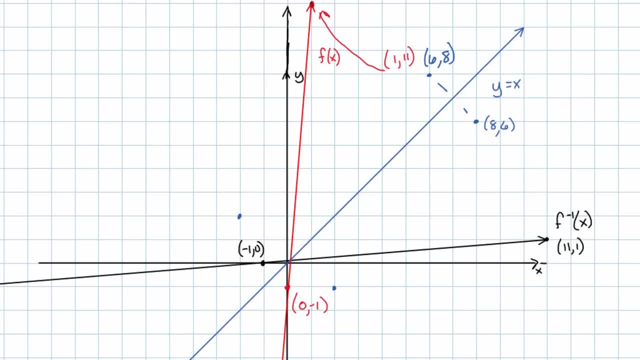 on the opposite side of y equals x, they will have opposing uh, x, x and y values and keep graphing the wrong one there, but twice actually. so, for example, this point right here is: x equals two, y equals a negative two. this point right here is: x equals the negative two, y equals two. and their mirror images about this blue line. okay so. 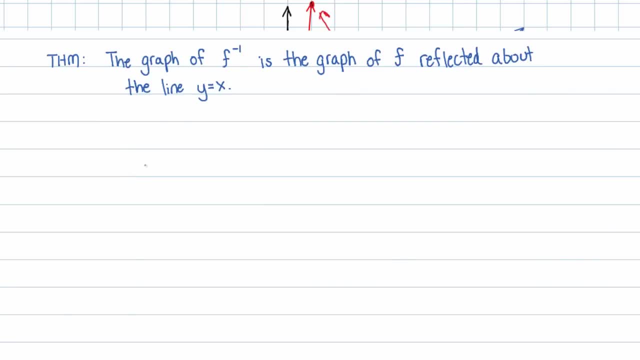 it turns out that the graph of f inverse is just the graph of f being reflected about the line y equals x. let's do a simple example that doesn't involve an actual given function. let's just say somebody comes up and gives you this graph of a function. 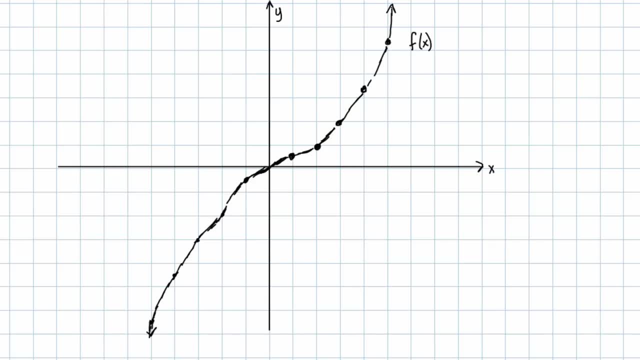 suppose somebody came along told me this is the graph of my function f. now what i want to do is graph the line y equals x. so this is y equal x and y equals a magneticgradive sum. and what i want to do if we laying total this: 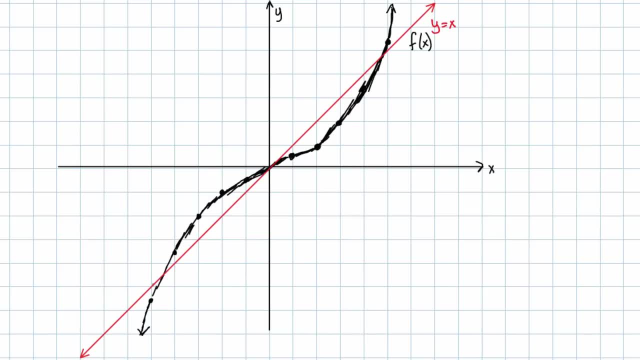 equals x, and if you probably notice, i just readjusted that curve because i kind of did it incorrectly, but anyway, so the black curve is some function f of x, and then i go ahead and graph: y equals x. now, if i want just a quick and dirty graph of this, of the inverse- and i'm not really 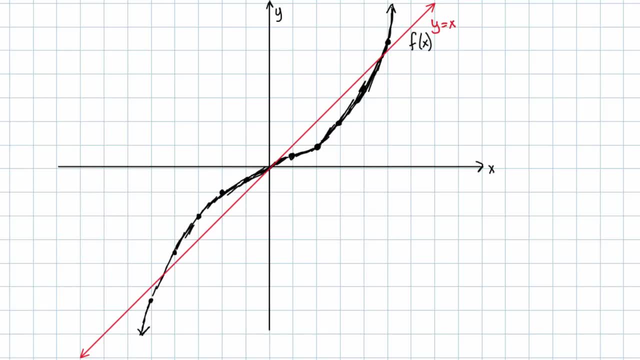 concerned about being super exact. i'll go ahead and just maybe choose a different color, because it'll get kind of confusing if i don't and it's going to be the mirror image about this red line. so, in other words, like over here, it's going to do something like this. it's going to do this. 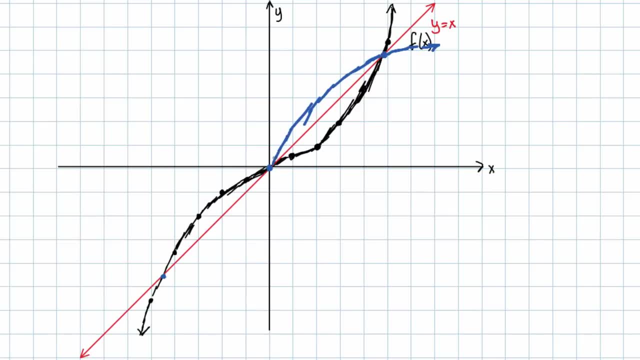 i want to come bow back in a little bit here. i know i'm doing a kind of a messy job, but it gets the point across right. it goes back around here- not the best again kind of a little messy ol and something like that. so the blue curve is something like the inverse function and that's. 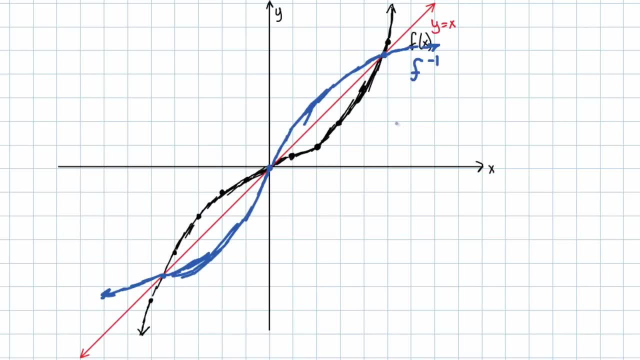 a quick and dirty way of graphing the inverse function. it's really just a very nice way to do things, because the fact is that you know whatever x, y value this point has, you swap them. it'll actually be right here for the inverse function. so very nice way to plot these. 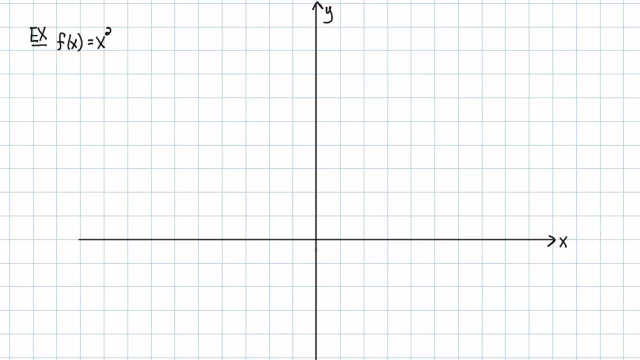 but that leads us to a kind of an interesting example as well. let's go. let's go ahead and graph f of x equals x squared. so when x is 1, y is the output's 1, when x is 2, the output's 4, and when x is 3, the output is 9 up here. so i'll just same thing with 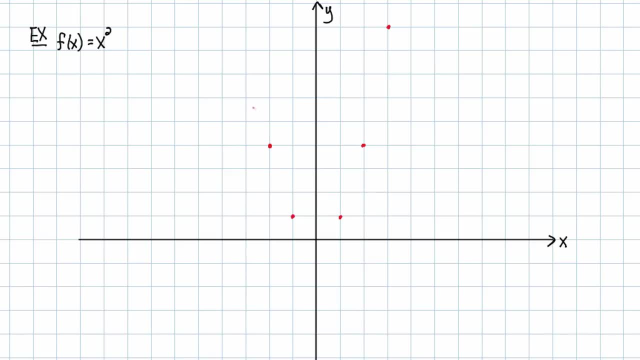 when x is negative 1, y is 1, when x is negative 2, y is 4, and when x is negative 3, y is 9, and then we go ahead and connect the dots right. it's it what's going to be interesting about this, and i'm going to go ahead and label those points. 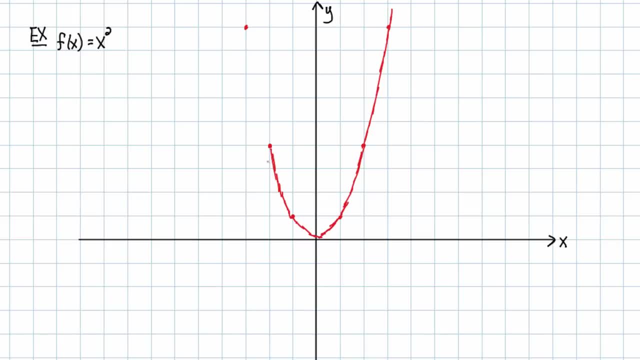 when you watch the last lecture on determining whether something's a function or not. uh, or actually i think the last lecture i did was on function notation, but i've talked about how to determine whether something, whether a function, is invertible or not, and i have mentioned that when you have an even power, it generally means it's the function's not invertible. 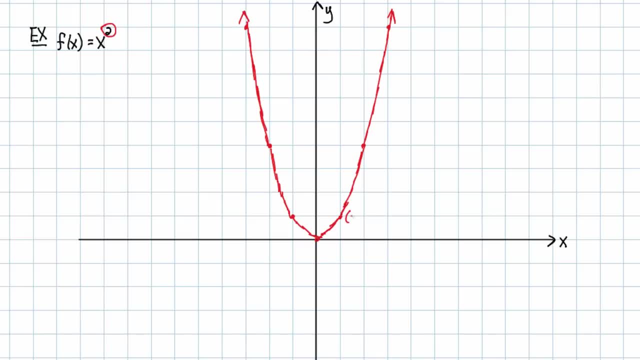 and here's why this function goes through 0, 0, it also goes through 1, 1, it goes through 2, 4 and 3, 9, so it's inverse. i'll do that in blue. should go through 0, 0, 1, 1, 4 comma 2, 1, 2, 3, 4 comma 2. 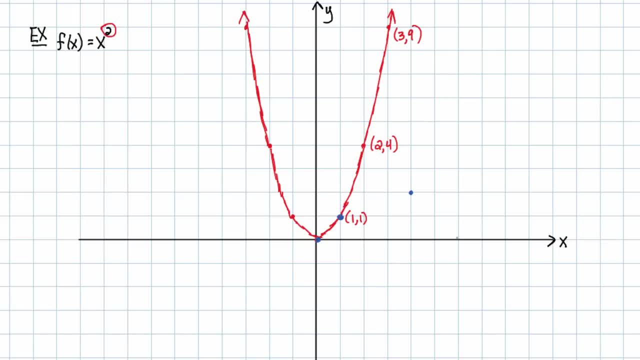 and 9 comma, 3, 5, 6, 7, 8, 9, up 3, so it should go through 0, 0, 1, 1, 2, 4 and 3, 9, so it should go through 0, 0, 1, 1, 2, 3, 4 comma 2. 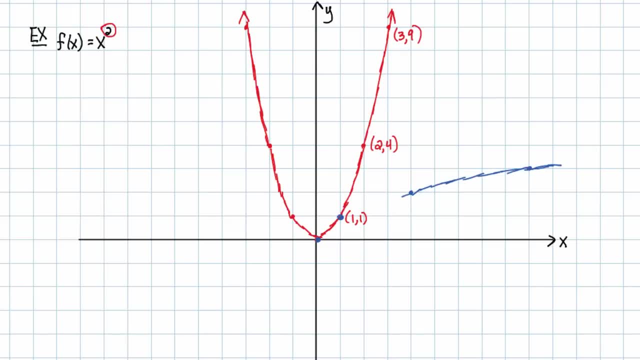 it should look something, should start to look something like this again, freehand drawing this. actually it would be above this red curve in this area, but it doesn't matter, so let me label those points. that's that's nine comma three and this is four comma two. 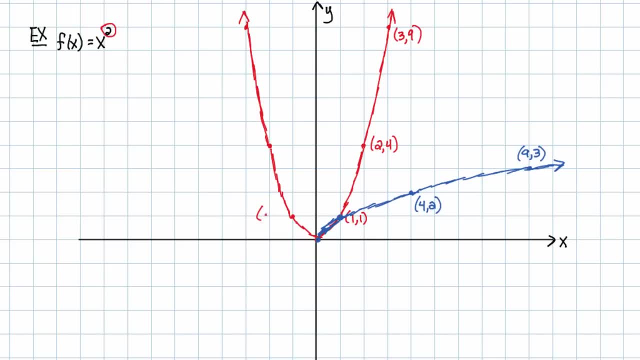 but remember for this parabola there's also these values over here: x equals to negative one. that's not how you spell. negative one y equals one, x equals a negative. two y equals four and x equals a negative. three y equals nine. so let me plot the opposites of those points. 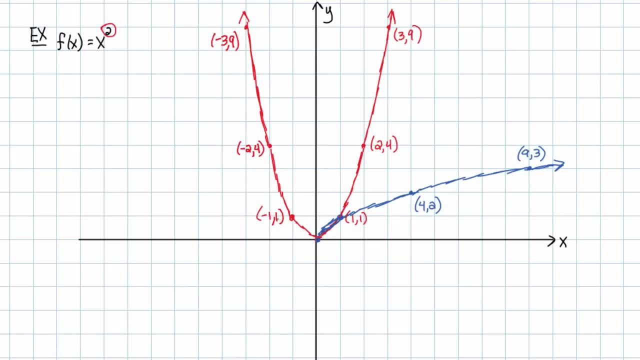 so in other words, swap the x and y values. uh, so for this first point here, swap them. i'll plot: x equals one, y equals negative one, x equals one, y equals negative one is right there. so one comma negative one, and then four comma two negative two. so one, two, three, four comma negative two is right. 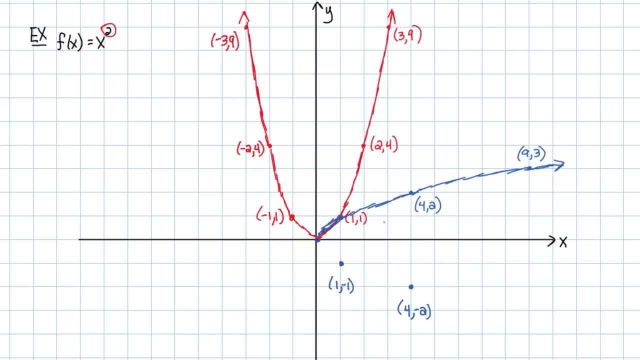 here you can already kind of see the shape. and then nine comma, negative three. nine comma one, two, three down you can see the shape. it's going to be a parabola. it definitely is a parabola, but it's on its side. i'll finish this out really quickly. 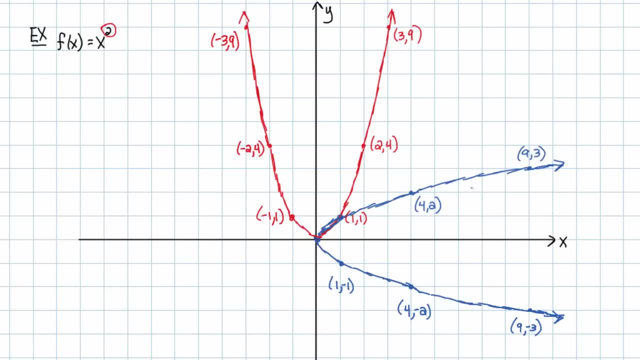 and the question is: is that a function? is that blue curve a function? and the answer is no, it doesn't pass the vertical line test right. so that means f was not invertible or not one to one. is there an easy way to determine whether a function is not invertible? well, if you have. 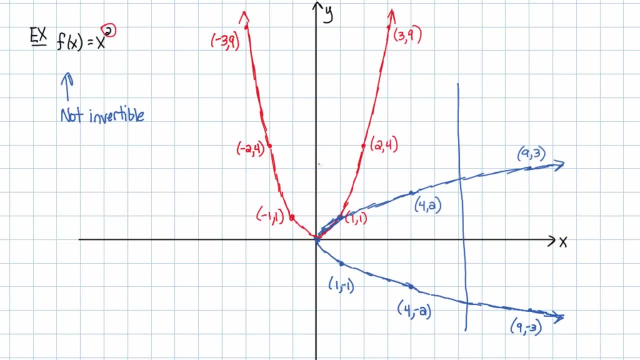 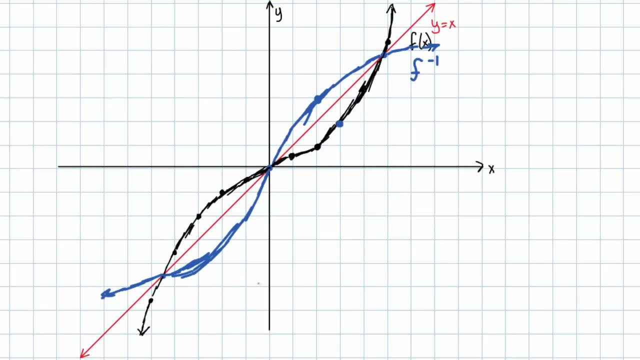 the graph of a function. super easy, all you want to say. you know a function is invertible. if, when you- uh, how do i say this? if every y value, like this y value right here, leads to only one x value, okay, so notice this y, this height right here, hits the. 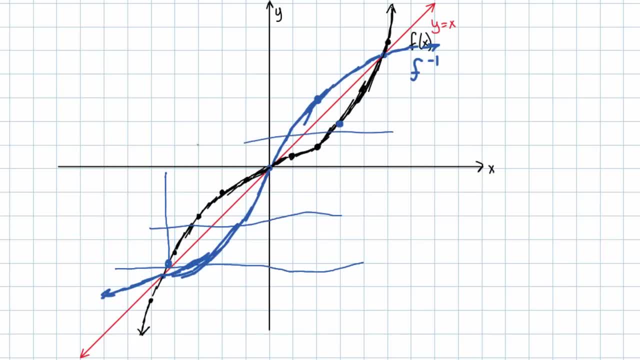 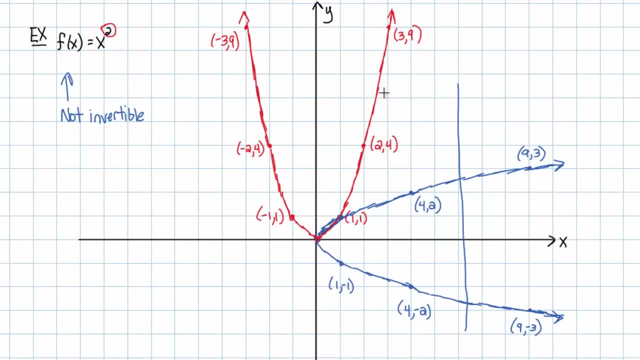 graph only once. this height right here hits the graph only once, and so on, so forth. so, in reality, to test whether a function is invertible or not, you can say: you know, a function is invertible. if a function passes the or is invertible, you draw a horizontal line. if you hit, if that horizontal line. 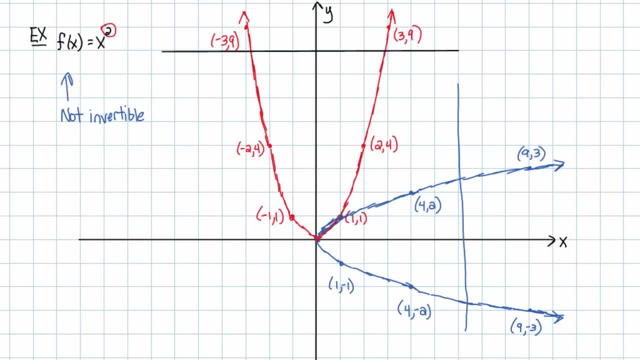 if any horizontal line you draw hits the graph more than once, it is not invertible, because what happens when you take the inverse is that, well, your domain and range swap, and that means that if you have two different x values that lead to the opposite direction, you're going to have a. 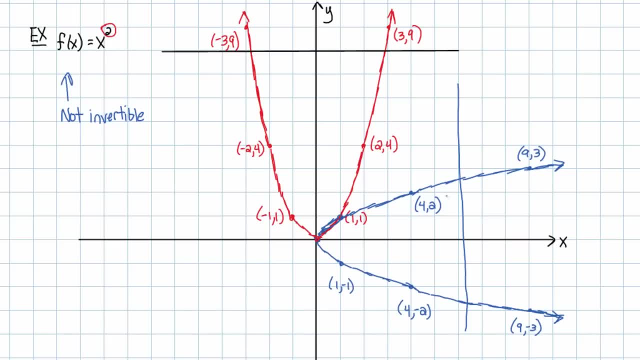 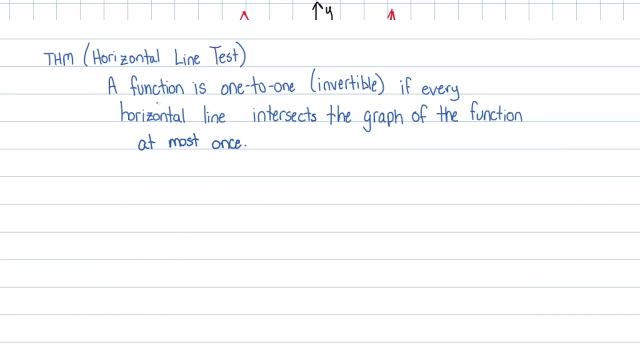 same output. well, when you try to find the input inverse, like in this case, you have one input that leads to two different outputs. that's a bad thing. so let's go ahead and write that down as a theorem. it's the horizontal line test. just like to find out if you have a function. 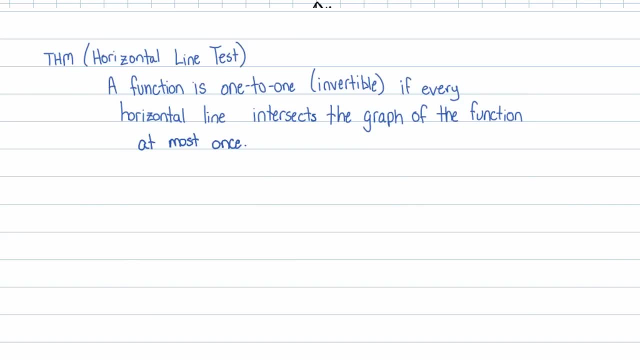 if a graph represents a function, you usually do the vertical line test. well, if you know that your graph represents a function and you want to know if it's invertible, do the horizontal line test. a function is one to one or invertible if every horizontal line intersects the graph of 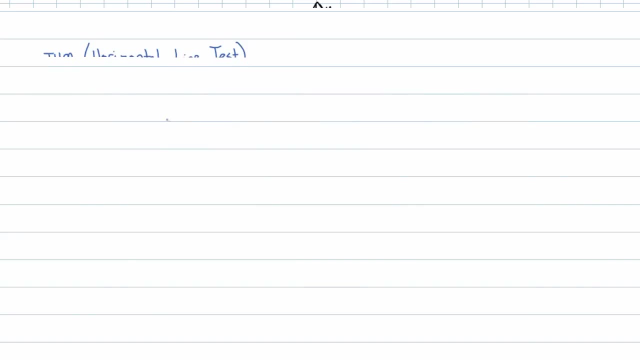 the function at most once. so at this point i could just draw up a quick few examples like this. this here is a function- don't get me wrong, this is a function f, but the fact is it doesn't pass the horizontal line. so while it's a function, it's not invertible. 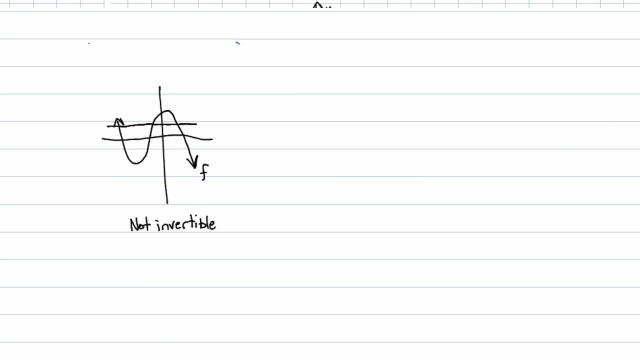 it's not invertible. it's not invertible, it's not virtual right now. so notice that each input leads to its own output, right, all these inputs lead to outputs. however, the output, of whatever height this is, leads to three different inputs, and so it's. that means that. 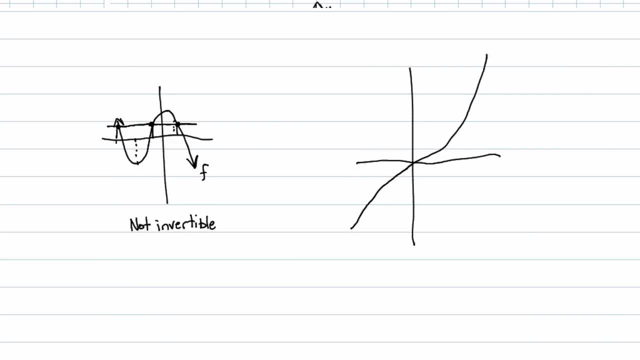 when we try to find the inverse, we'll. we'll not have a function. that's a function f and it does have an inverse, because every single horizontal line i draw crosses the graph at most once. so there you go. there's, i mean it's, it's pretty much just. 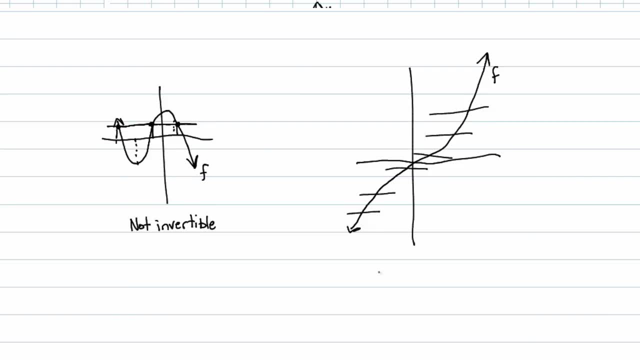 that easy. most students find this topic to be pretty straightforward. now, the last little bit that i want to talk about is more of a recollection of why i complain about the current function notation. so let me give you a simple example. now, remember we write f of x, let's just say. let's say f of x is equal to 1999. 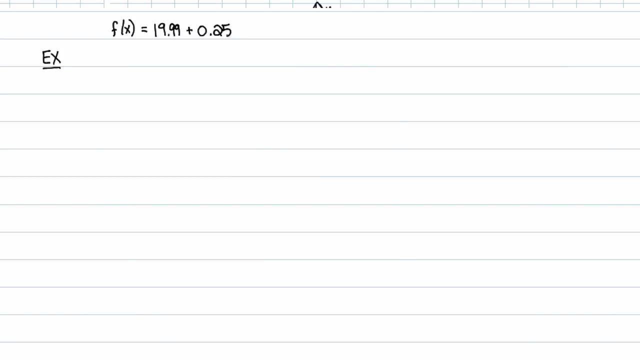 plus 0.25 x. well, whenever we find the inverse, i like it written as f inverse of y is equal to okay, and it would in this case it would be actually y minus 1999 over 0.25, and i don't know if you can see that that might be at the top of your page. 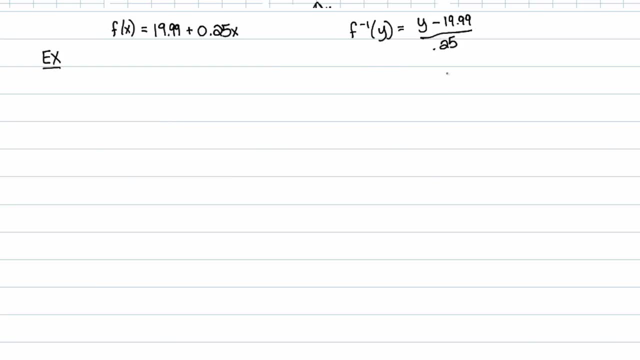 i'm not 100 sure, but it doesn't matter. i'm going to do it again. but just to let you know that most textbooks insist that that be written as f inverse of x and they insist on swapping variables and, as we've seen in this lecture, it's really useful to swap variables when you want a graph. 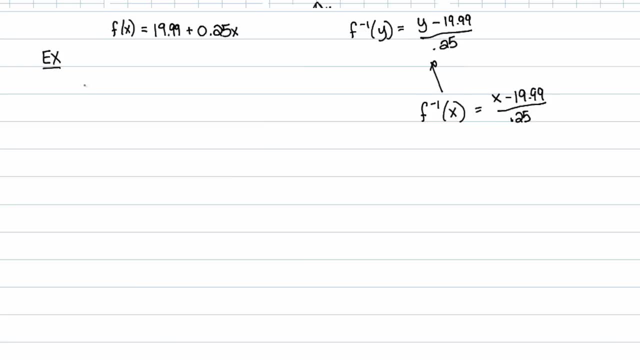 but otherwise it's pretty useless, especially in applications. so suppose that you rent a u-haul and i've given this application way back early in my lecture series. but suppose you rent a u-haul and it costs $19.99 plus 25 cents a mile. 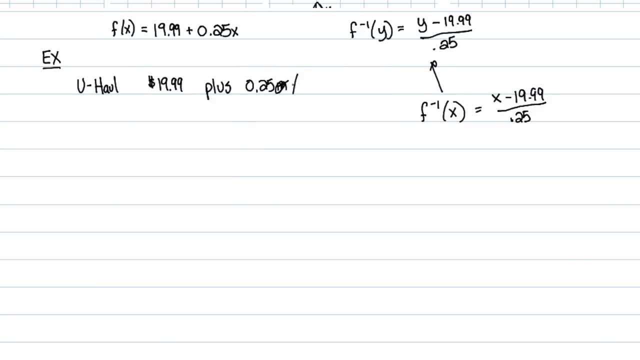 oops, i already. i, i think, in math, so 25 cents per mile. so therefore, if you want to create a cost function in terms of the number of miles that you've driven, it would be $19.99 plus 25 cents per mile, so so. 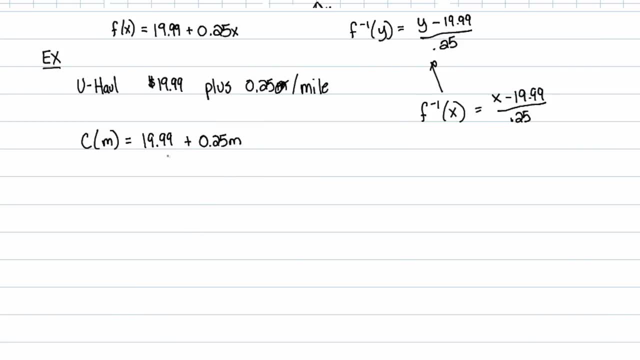 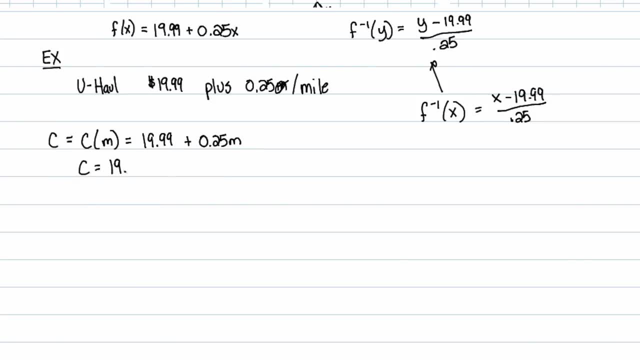 actually. so c is equal to $19.99 plus 0.25 m. this whole business where f of x is always equal to y, that's bs. you could choose any letter you want, honestly, so let's solve this for you. cm enough. actual integral f. 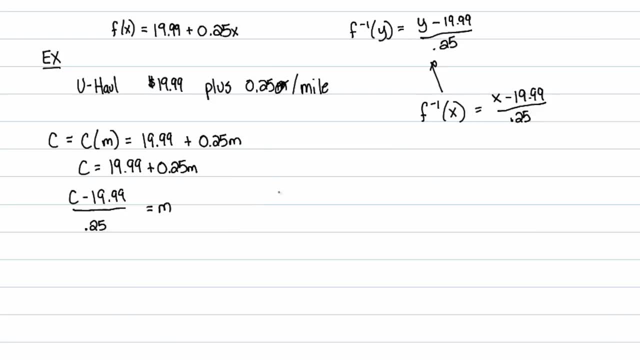 that m talked to hour 0.25, 0.25, 100, 9, 0.25, 0.25, 0.26, 0.27, 10, 1, 3 minus 1999 over 0.25, and I know that C inverse is supposed to be the input. 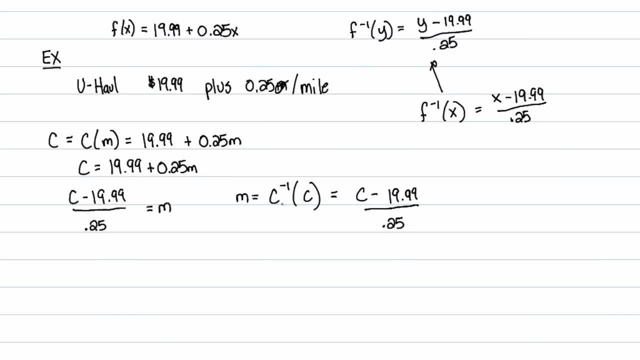 value now because I use the same letter. it'll look kind of confusing, but don't think these, don't let it confuse you. the fact is the inverse function. we're going to plug in a cost and I'm going to see how many miles my output is the